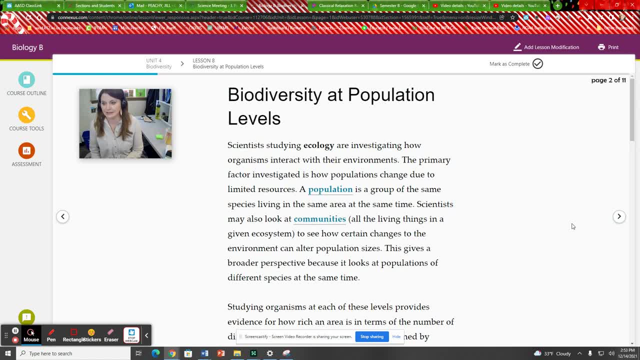 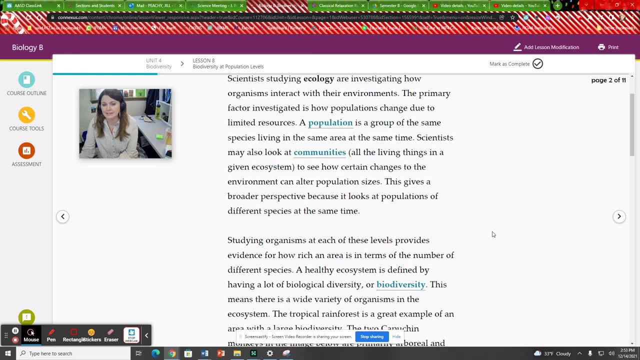 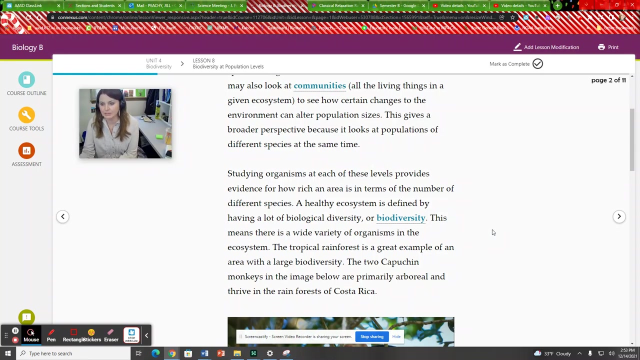 This is something that scientists are very interested in. They're also interested in how different populations kind of affect each other. So looking at whole communities- because sometimes we have changes in one population that has an impact on another population- it gives us kind of a broader perspective of what's going on. And then we talk about something called biodiversity. So biodiversity is the variety of organisms that are found in an ecosystem. And a healthy ecosystem is a healthy ecosystem. ecosystem is biodiverse, As I mentioned earlier. some ecosystems are more diverse than others. just naturally, What we want to have is to maintain the natural level of biodiversity within that specific ecosystem. Some ecosystems that are extremely biodiverse include tropical rainforests. and coral reefs. So we have our terrestrial kind of most diverse of all ecosystems, and the coral reefs being the aquatic most diverse of all ecosystems. What do you find here? You find a wide variety of different plant life. You find a ton of different types of animals. There are mammals like jaguars and rats. There's birds like toucans and hornbills. There are thousands, millions of different types of insects. The canopy of the rainforest has over one million insect species all by itself. Many of the rainforests are very diverse, So we want to have a wide variety. 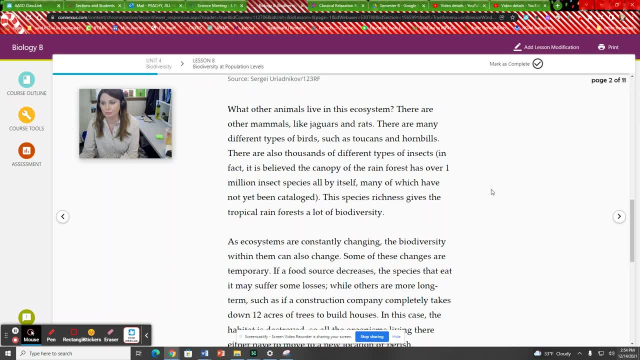 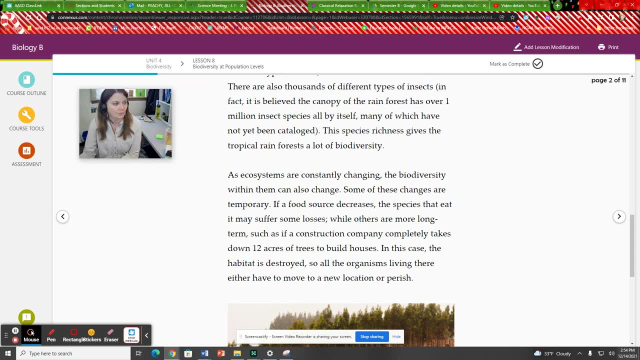 of species, some of which have not even yet been cataloged. The species richness gives the tropical rainforest lots and lots of biodiversity. So I have on here what can cause changes in biodiversity, and are those changes temporary or permanent? So ecosystems are constantly changing and biodiversity. 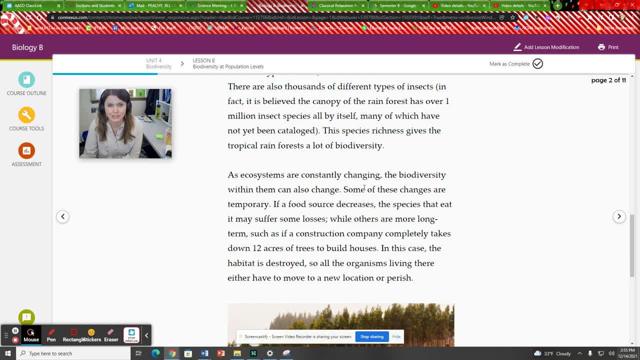 changes with them. Some of them are just temporary seasonal changes, for example in biodiversity, or changes that have to do with natural conditions, So, for example, we might have more vivera than we. natural cycles of drought, for example, can be temporary changes in biodiversity. If a food source decreases, the species that eats it may suffer losses, while others are more. long-term Deforestation, for example- clear cutting of forests- can permanently decimate biodiversity in a specific area. All the organisms that lived here either have to move someplace else or they. 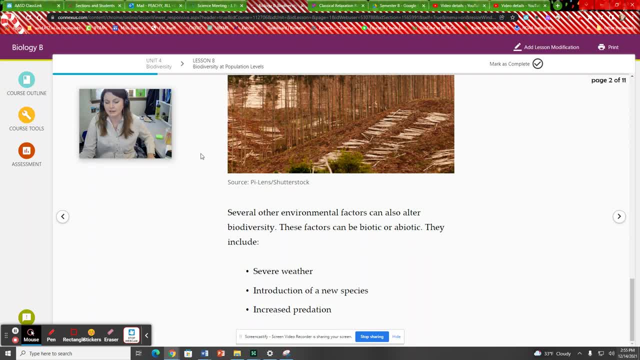 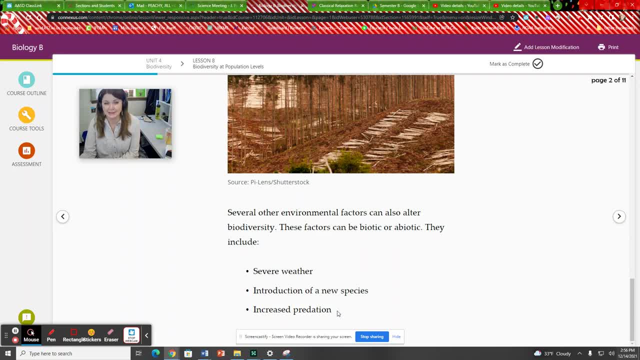 the species that eats it may suffer losses. If a food source decreases, the species that eats it may suffer losses, wreak havoc on biodiversity In this area. right now, we are losing all of our ash trees. We have an introduced species, an invasive species, the emerald ash borer. that is just. 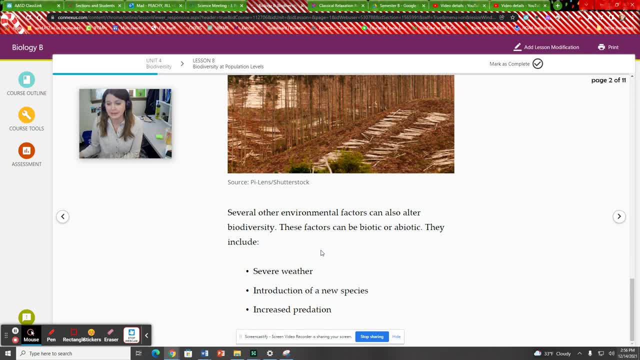 decimating our ash trees all throughout the United States, And this is just one example, excuse me, of how introducing a non-native species can wreak havoc on an entire ecosystem. You lose the ash trees, ladies and gentlemen, and all the animals that roost in those trees. and live in those trees, the squirrels, the birds that live there, the birds that feed upon the insects that live in them- they're all going to suffer the consequences of the loss of the ash trees. You also can have increased predation that can cause changes in biodiversity. 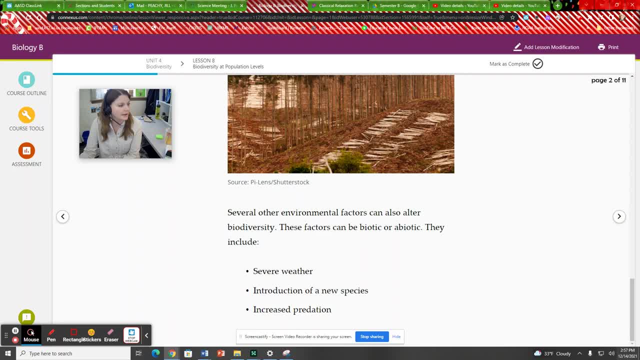 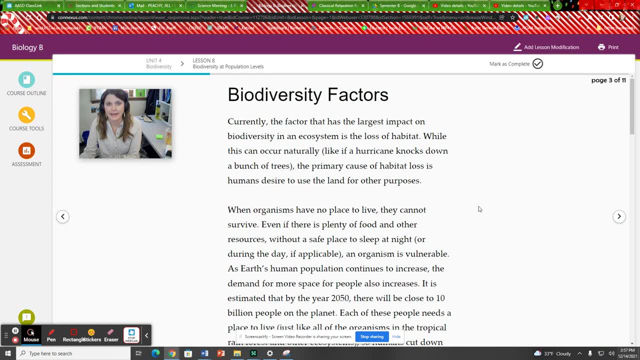 These are just some examples. We'll talk about a few more examples coming up in the next part of the lesson. So it says here that the largest impact on biodiversity is habitat loss And the largest contributor to habitat loss is people. People cause most of the habitat loss in all ecosystems, And this is due to humans' desire. 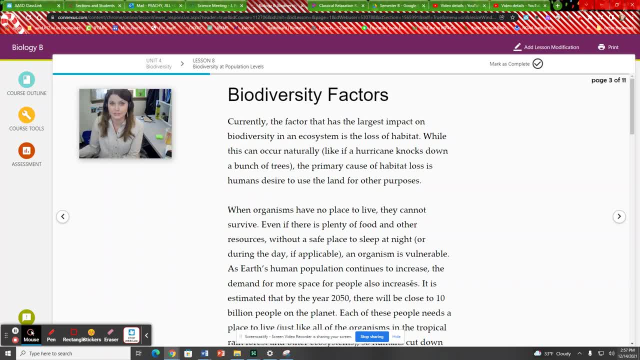 to use that land for other purposes. They clear-cut areas of forest to use for agriculture, Or they take an area that once was an ecosystem, a prairie for example, and they construct a, a new housing subdivision there, right? So organisms then that lived there have no place. 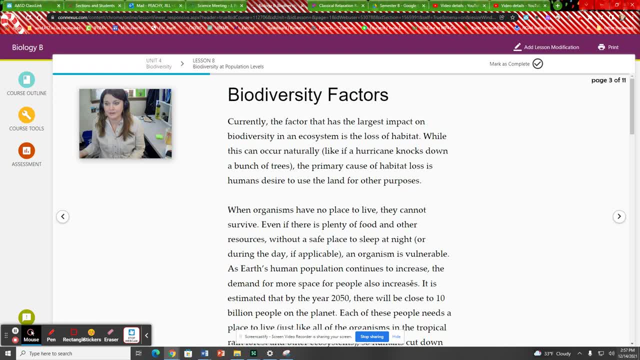 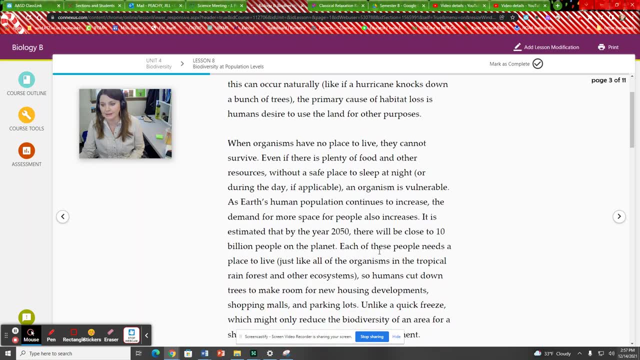 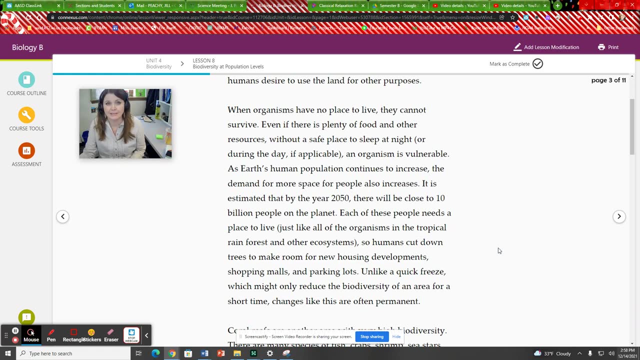 to live, They can't survive. They may have food and other resources, but they don't have a place to stay. And if they don't have a place to call home, that organism is vulnerable and can suffer losses. As it goes on to talk about human population and how it is, it is estimated that by 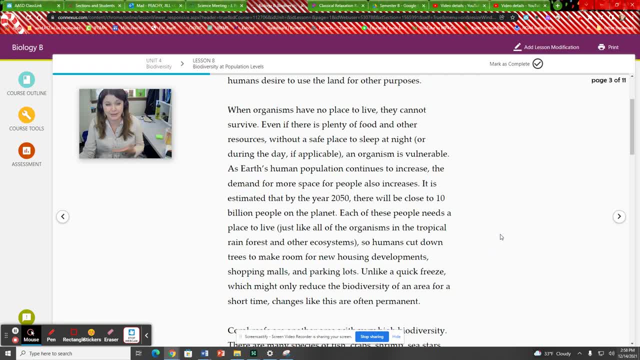 the year 2050, we will have close to 10 billion people on the planet, which I know. in a previous lesson they talked about 10 billion people on the planet And they talked about 10 billion people as being the potential carrying capacity of humans on Earth. I think we'll kind of see if that 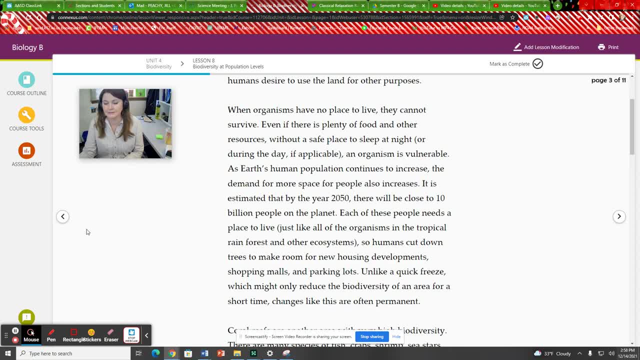 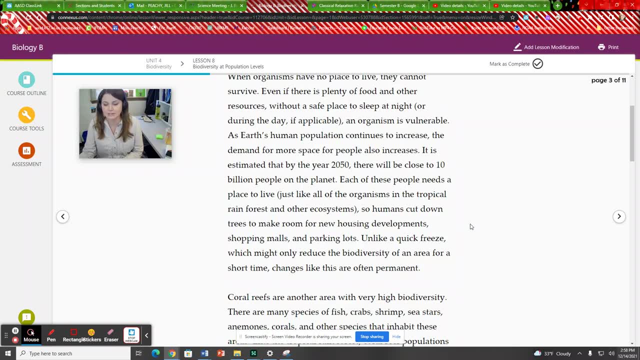 actually holds true. But all of these people need a place to live, just like all the organisms in the tropical rainforest or any other organisms. So humans have to cut down trees to make room for new housing, developments, shopping malls, parking lots, et cetera, et cetera, et cetera. right. 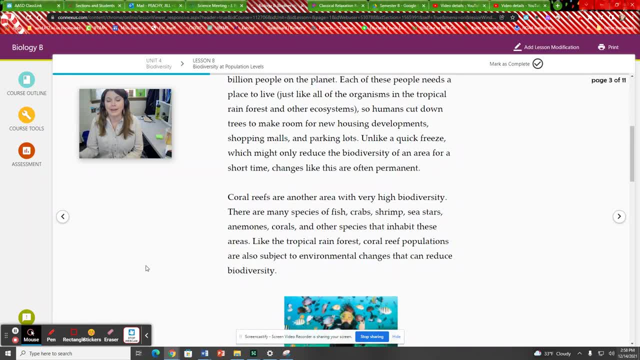 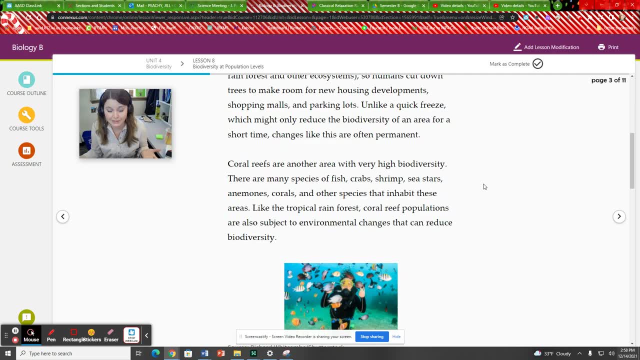 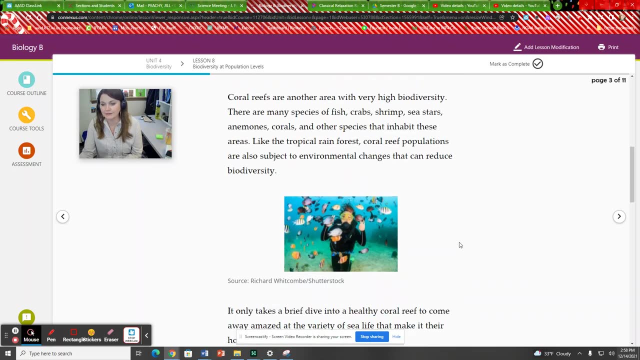 And so we just continually take from other habitats to be able to live. It also talks about how coral reefs, which, again like the rainforests of the ocean, they're highly biodiverse, and that there's a lot of problems with the coral reefs. that's also impacting the 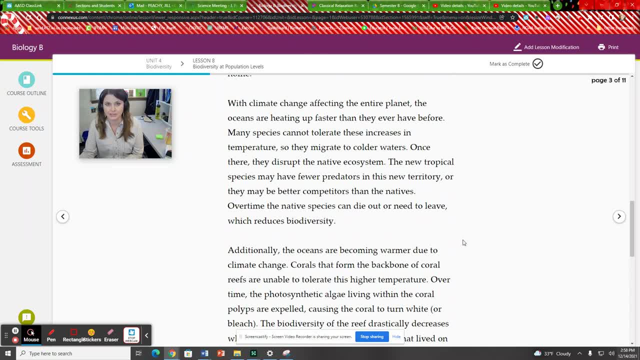 biodiversity. In this case, it is discussing climate change and how climate change impacts coral reefs. We talked a little bit about this- I don't remember which lesson it was just more recently here- how corals have an algae that lives within the coral. They actually live in this mutualistic relationship with algae. the zooxanthellae And the algae are kind of temperamental. They need a very specific temperature to be able to survive and thrive, And if the temperature of the water gets too warm, the algae will leave the coral. 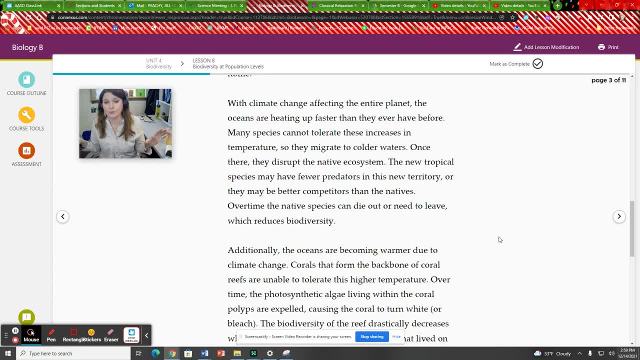 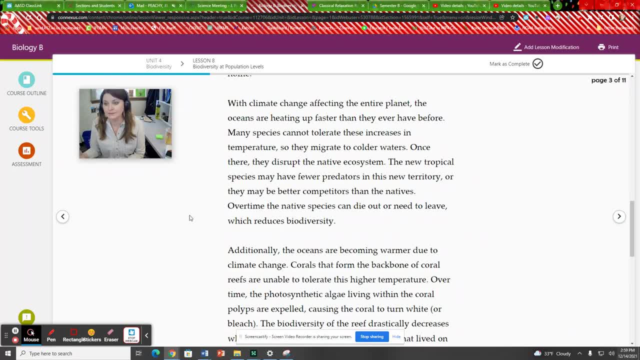 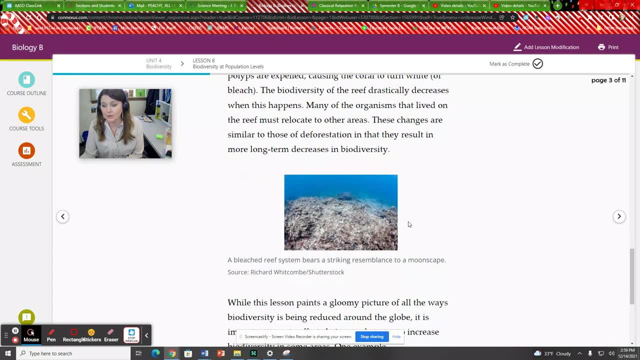 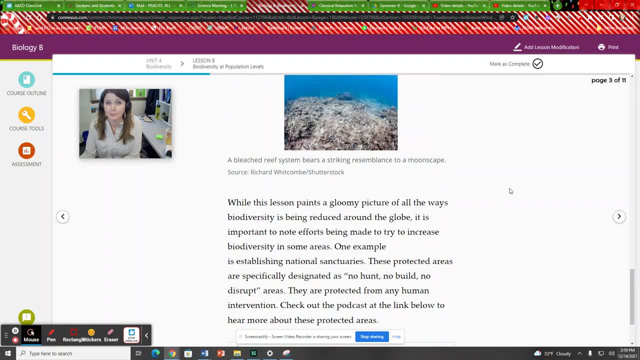 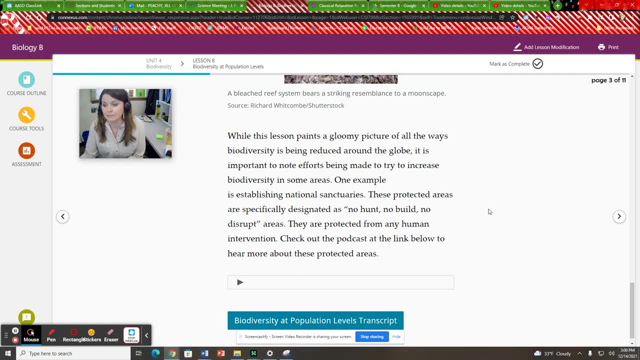 the environment. here We're having a lot of devastating effects And I think we're all kind of more aware of this now And hopefully in the future. today and in the future we can make some steps to mitigate the damage that we are causing to the environment. So, moving on to the 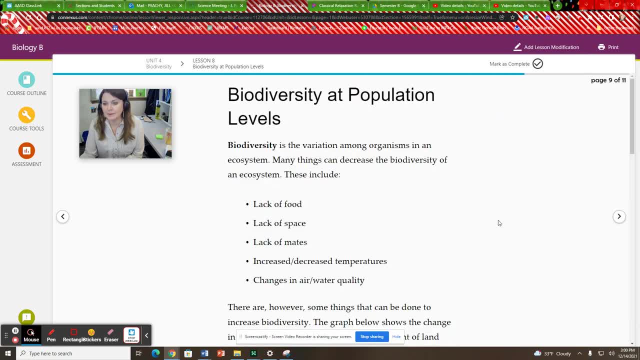 last one, we're going to talk a little bit about the coral reefs And I think we're going to talk a part of this lesson. it talks a bit more about biodiversity and I just wanted to include this because it talks a little bit about a few more things that affect. biodiversity, a lack of food, lack of space, lack of mates, increased or decreased in temperature, changes in air or water quality, all of those things kind of help, they kind of like hurt. I guess biodiversity it's not even an including, like competition for like invasive species and stuff in this list. 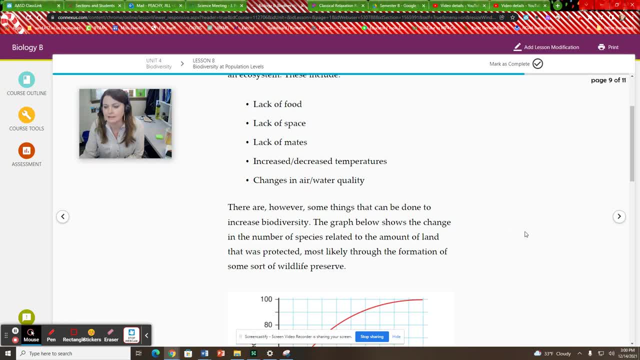 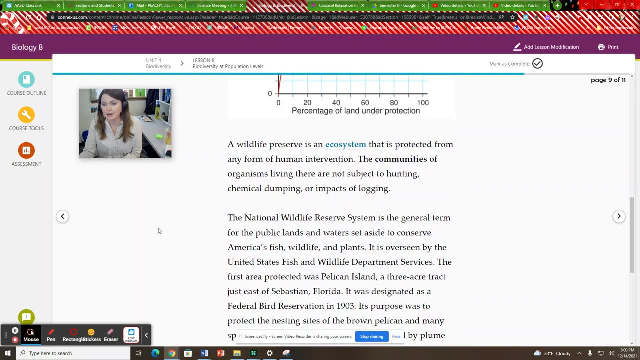 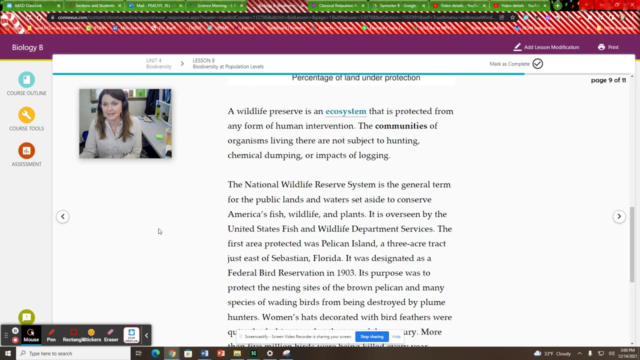 so both lists are somewhat incomplete, but all of those things are affecting biodiversity. so how can we help, what can we do to increase biodiversity? and so they talk a little bit about one of the things that we can do. we can set up wildlife preserves that are protected from any form of human intervention. here. 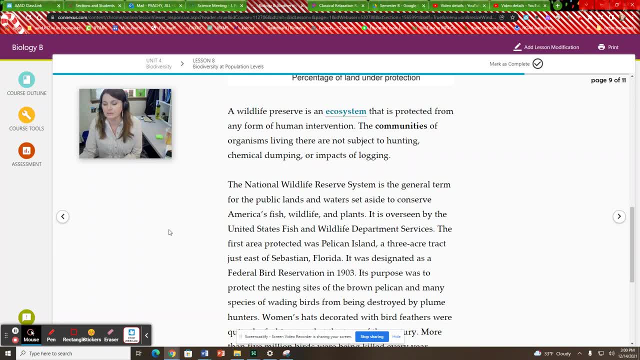 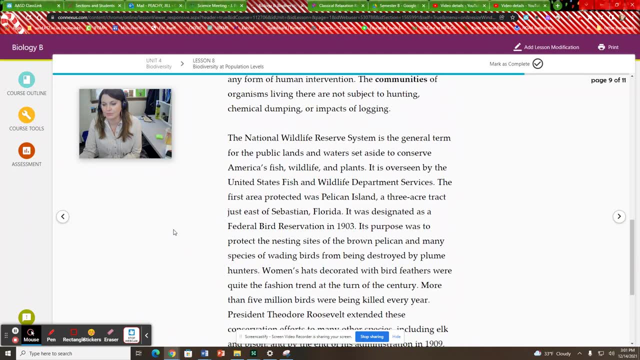 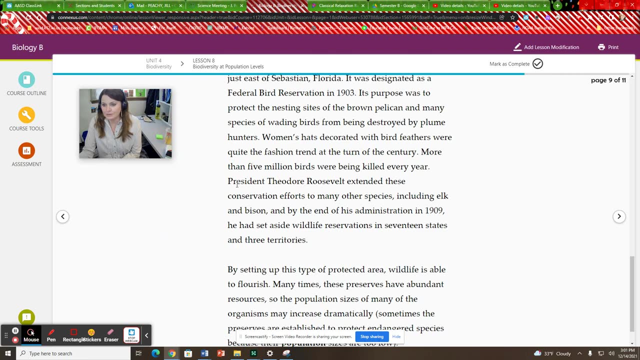 communities of organisms that live there. they're not subject to hunting, chemical dumping or impacts of logging, and it talks a bit about some of these wildlife reserves that have been set up throughout the country. Specifically, it's talking here about the efforts of President Theodore Roosevelt.